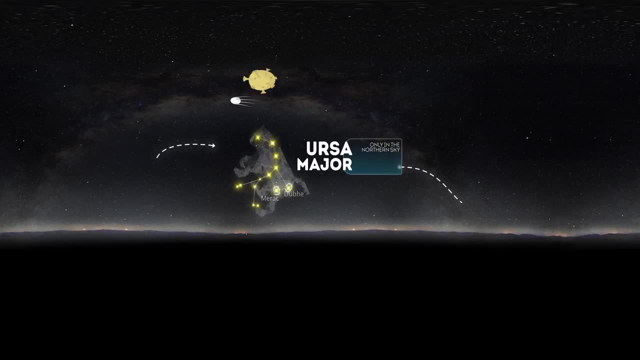 However, you should know that it can only be used to identify the Great Bear. It can only be found in the northern sky. What's interesting about this constellation is that many different civilizations saw it as a big female bear. Like this video if you have trouble seeing a bear shape in a bunch of stars. 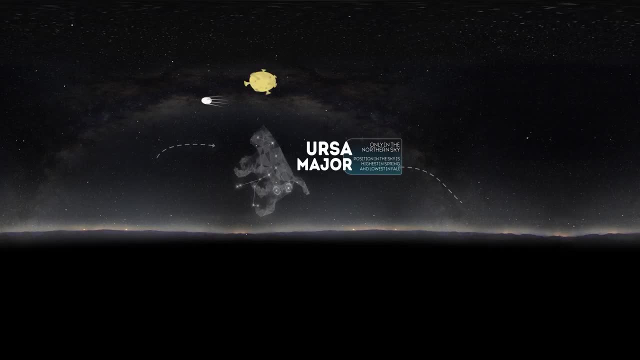 Its position in the sky is highest in spring and lowest in fall. The story goes that in fall, the bear looks for a place for its winter hibernation- Ursa Minor. Ursa Minor, also known as the Little Bear. Ursa Minor, also known as the Little Bear. 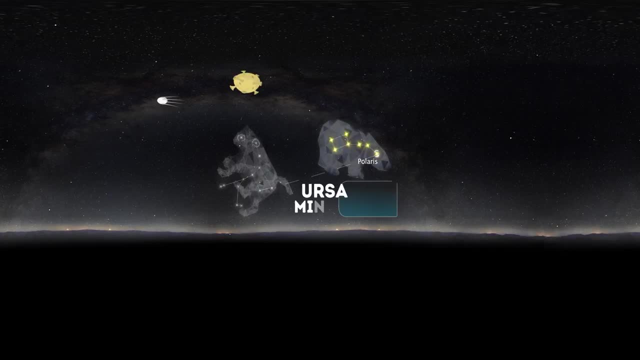 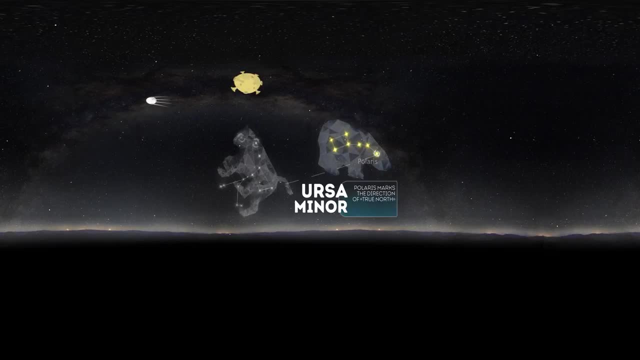 The main star in the constellation is Polaris, also known as the North Star. It marks the direction of true north for those in the northern hemisphere and the very beginning of the Little Dipper. Sailors use Polaris for navigation in the sea, before GPS, of course. 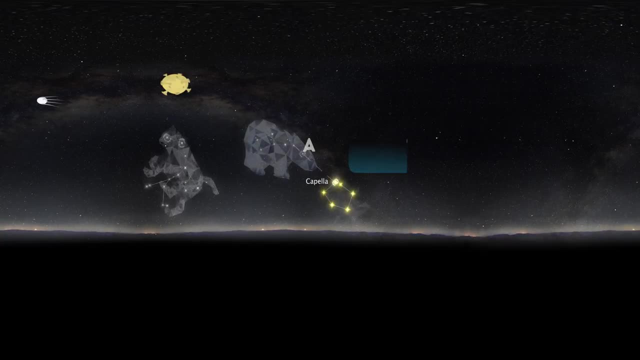 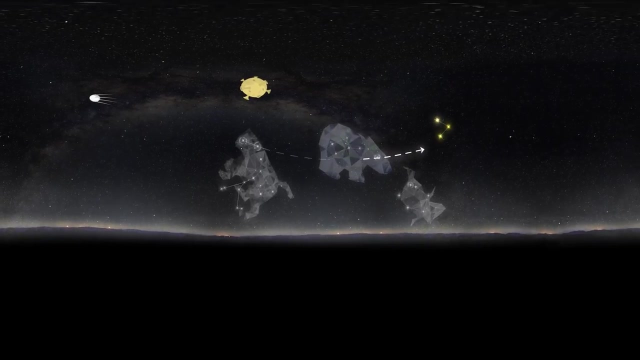 Auriga. Auriga is the Latin name for charioteer. In Greek mythology it is often associated with the Greek hero Erichthonius, who invented a horse chariot. Auriga is best seen in winter evenings- Cassiopeia. 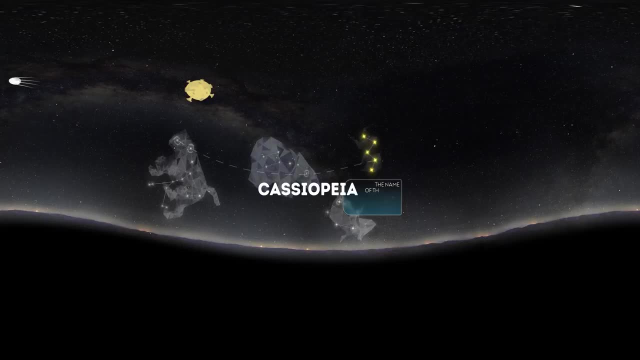 Cassiopeia is the name of the queen in Greek mythology. She was famous for showing off with her unique beauty Again. those living in the northern part of the planet are lucky to see Cassiopeia all year round, especially clearly from September to November. 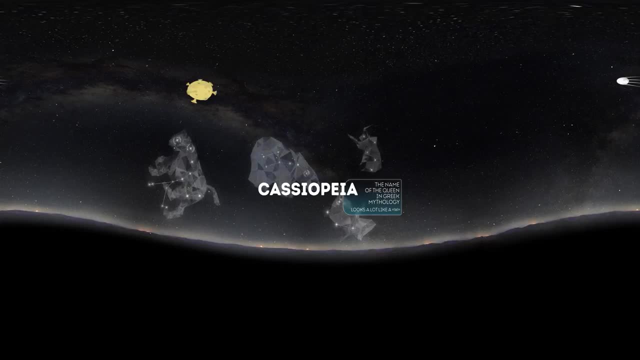 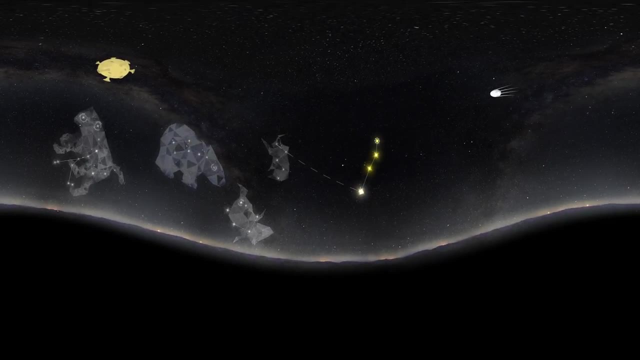 It is formed by five stars and it's easy to recognize because it looks a lot like a W: Andromeda, the chained woman. And here comes another beauty. Andromeda was a princess who told the sea nymph that they were less beautiful than her. 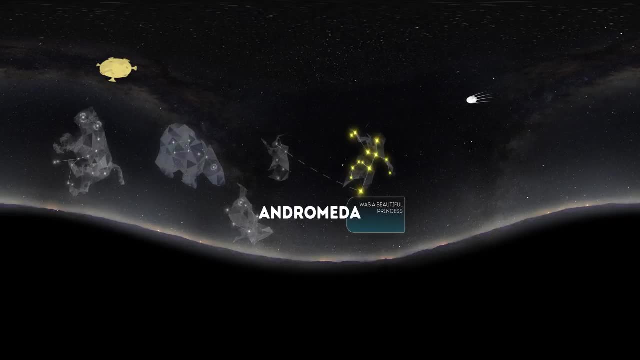 Wow. The nymphs couldn't take a blow that low and complained to Poseidon. The sea god didn't like that and threatened Andromeda's father to flood his camp, And the only way to save it was to sacrifice the daughter. Andromeda was chained to a rock but, lucky for her, Perseus came to her rescue. 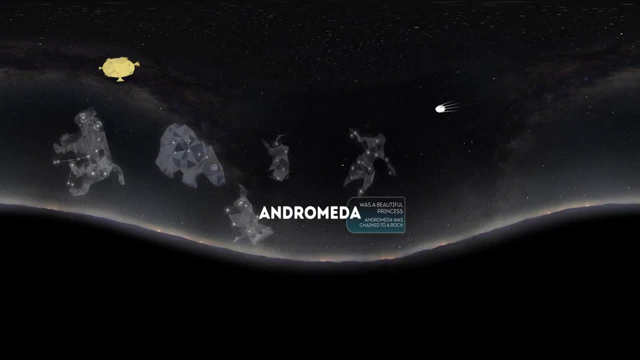 Ah, those crazy Greek gods. What are you going to do with them? huh, Formed by 16 main stars, the constellation does look like a person a little. However, it's quite hard to tell if the person is really that beautiful as the myth says. 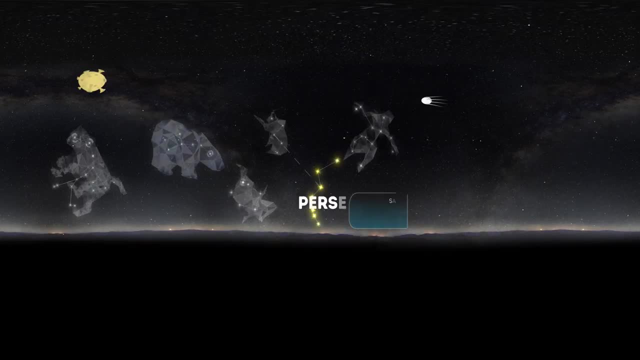 Perseus, Perseus, Yep, this is the same person. This is the same Perseus who saved Andromeda. He and the alleged beauty married and had six children. It is best viewed from August to March in the Northern Hemisphere. 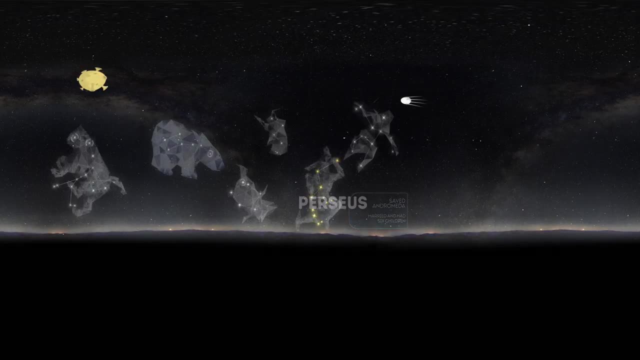 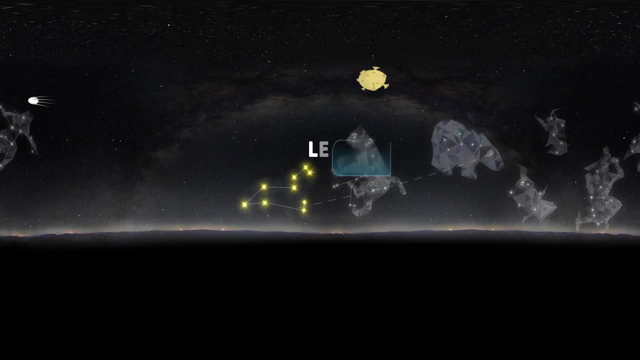 And in the southern part, you can see it in the middle of the spring. Leo: You must know this constellation as Leo on the zodiac signs. Leo is Latin for lion, the same lion that was killed by Hercules. Ooh, don't tell PETA. 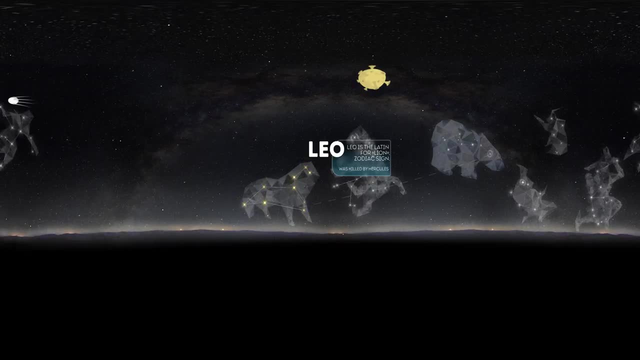 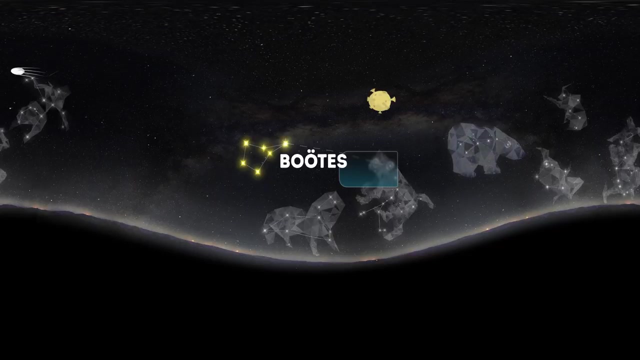 Just like Ursa, Major Leo was seen as a lion by various civilizations: The Persians, the Indians, the Turks and others. In the Northern Hemisphere it is best seen in May. Boötis, Boötis or Boötis or you know whatever. 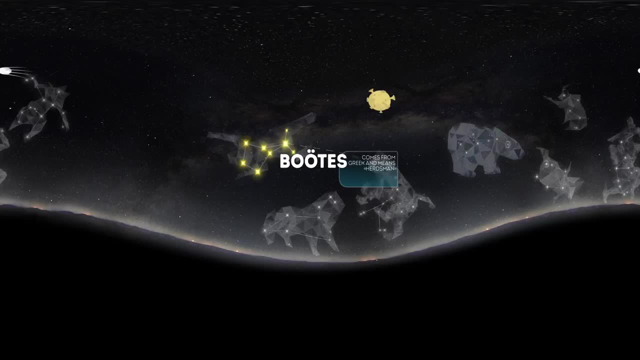 This strange-looking word comes from Greek and means herdsman. According to one of the myths, Boötis is Icarus, who got a secret recipe for wine. Icarus loved the drink a lot and later invited his friends to enjoy it too. 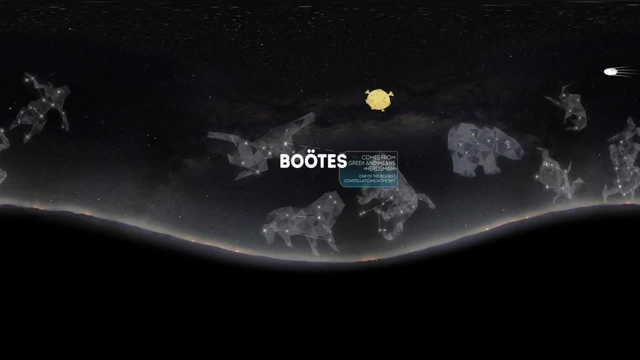 In the morning, the friends woke up with a terrible hangover and thought that Icarus had tried to poison them. They decided to kill him, So Icarus was placed in the sky. Wow, taking it a little personally, aren't we? 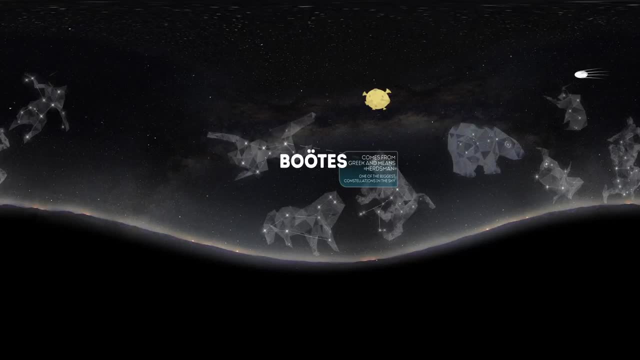 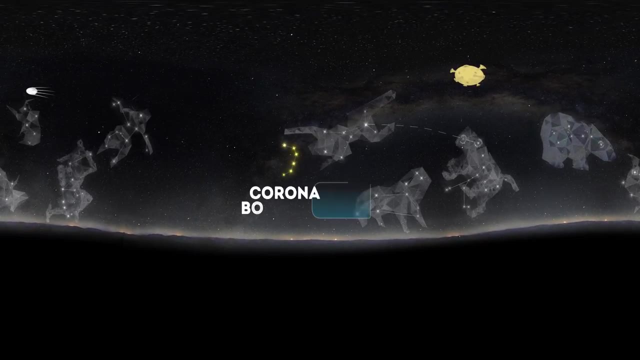 Anyway, Boötis is one of the biggest constellations in the sky. Corona Borealis, Again. Corona Borealis is the Latin for northern crown. In mythology, it symbolizes the crown that Dionysus presented to Adriani. 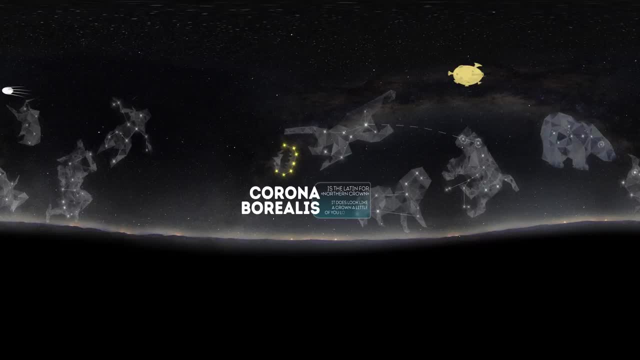 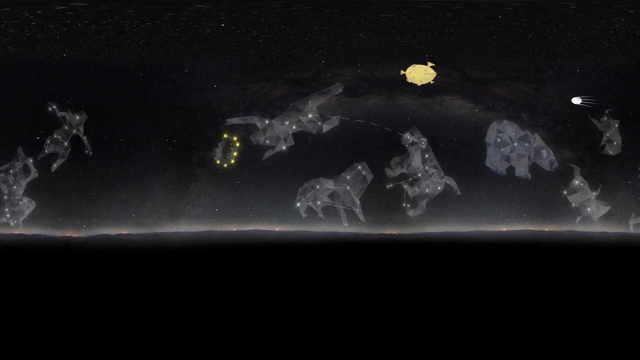 the princess of Crete. Well, we have to admit, it does look like a crown a little, if you kind of squint. Are there any other space-related topics you'd like to learn more about? Tell us in the comment section below. 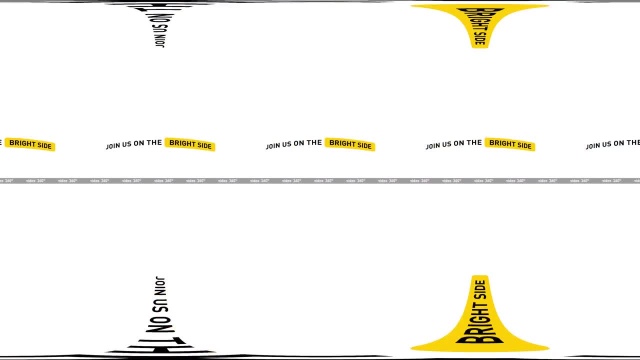 Be sure to share this video with your friends, to look up the constellations together, And don't forget to give us a thumbs up. See you right back here for more of the Bright Side of life. Subtitles by the Amaraorg community.